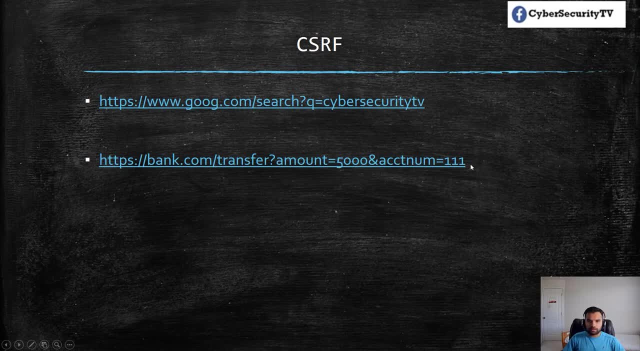 transfer five thousand dollars from your account to this one one, one account number. now, if you click on this, it may happen that your bank would, like you know, do this transfer, and I'm. this is just an example. of course you might have, like you know, some confirm button, or there are some. 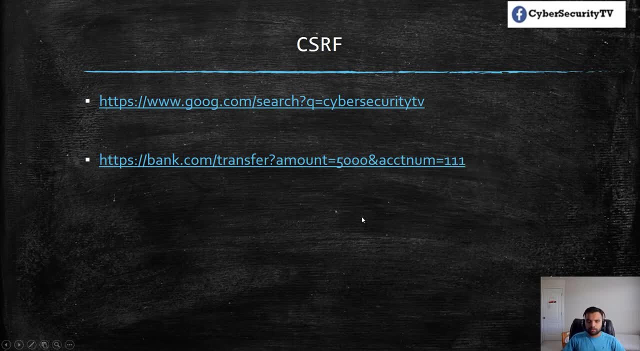 information, like multi-factor authentication, some unique code you have to put in. but let's just assume that- that there are some transaction on the website, for example like delete user. so there is a link which says delete user and the username and you click on it, that user is deleted. so similarly, that's. 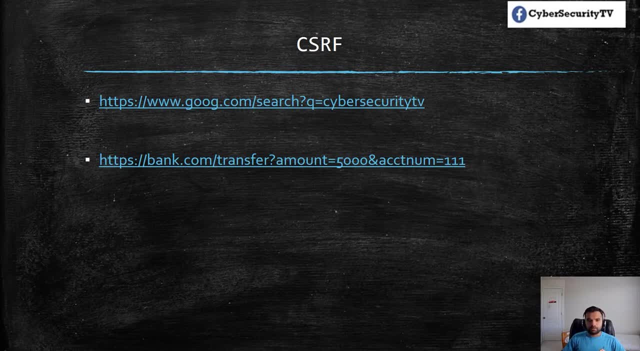 what the cross-site request forgery works. so when someone sends you this link, maybe, let's say, via Skype or Google chat or email, you click on it and and something bad happens which you don't realize. so why this is happening is because you don't realize. so why this is happening is because you don't realize. so why this is. 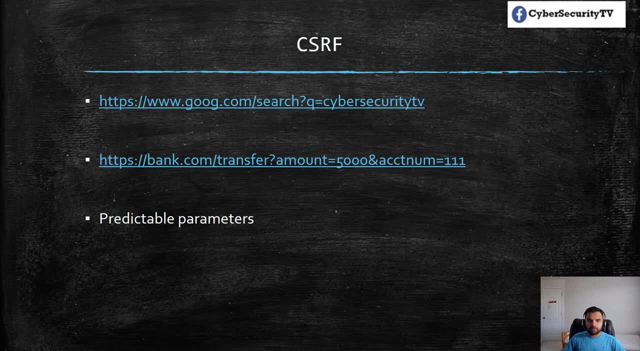 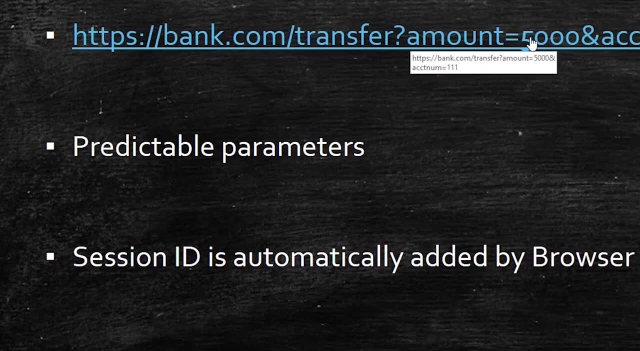 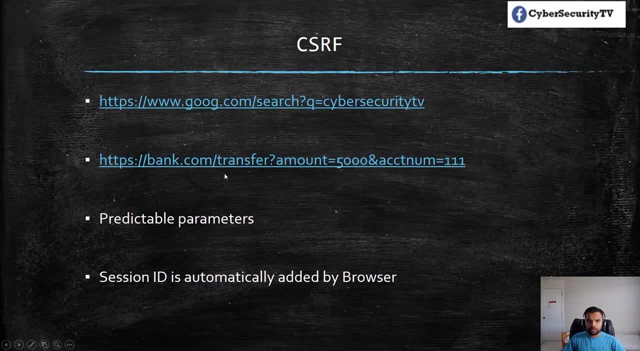 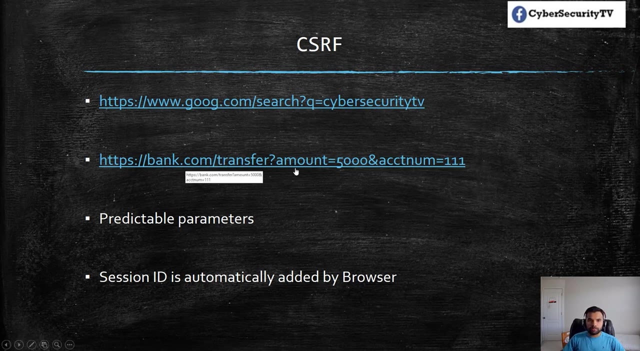 Facebook, right, and and let's say, there is a URL for create post and in, and one of the parameter is, like you know, the message and where I type the message. so I, as an attacker, know exactly what parameter that the website is looking for. so I would just create the URL with the message. whatever you want, I send it. 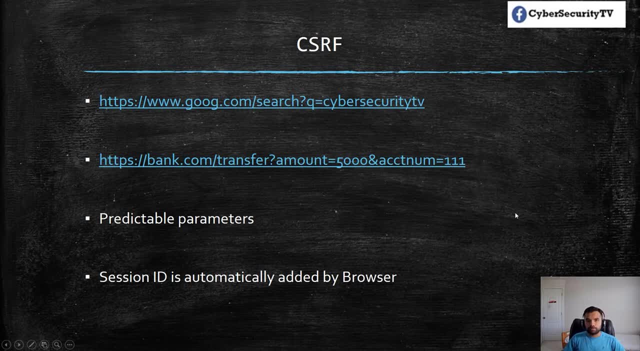 to you. you click on it and it gets to you and it will send it to you anytime it and it will execute, so it will post the message. however, you did not intend to do that. it was the attackers intention and behalf of the attacker. you posted that message on your wall and the and the most important reason for this, 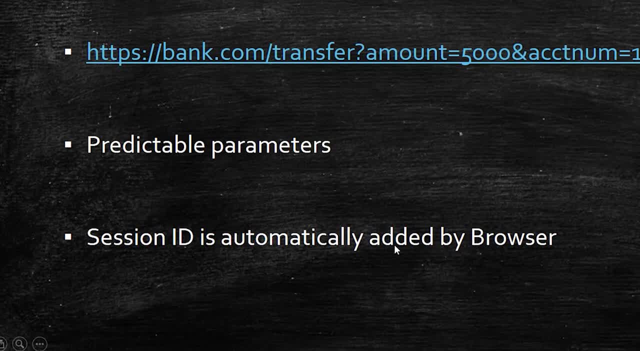 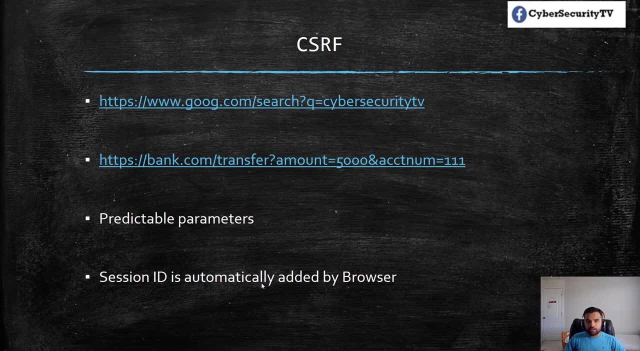 happening is session ID is automatically added by the browser, right. so when when you are logged into the Facebook in your browser- let's say Chrome- and when you click on this link, it automatically is open, opens up in the Chrome browser, and then Chrome browser will automatically attach your session ID in that request. 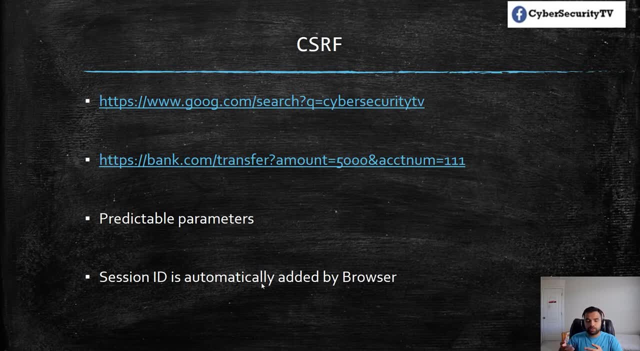 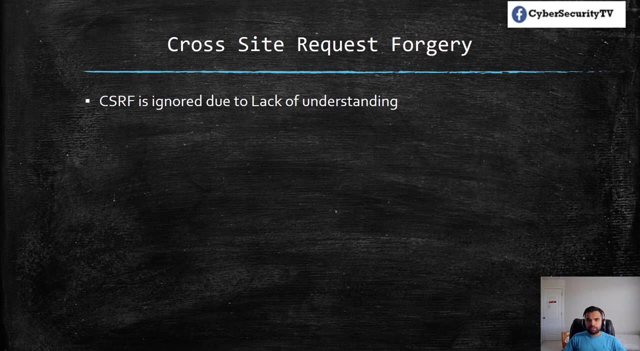 so it will not ask you, or whether you want to authenticate, or because you are already logged in, so it's gonna automatically transfer this amount to, or post the message on behalf of the attacker. now, CSRF is mostly ignored due to lack of understanding, because developers do not know. 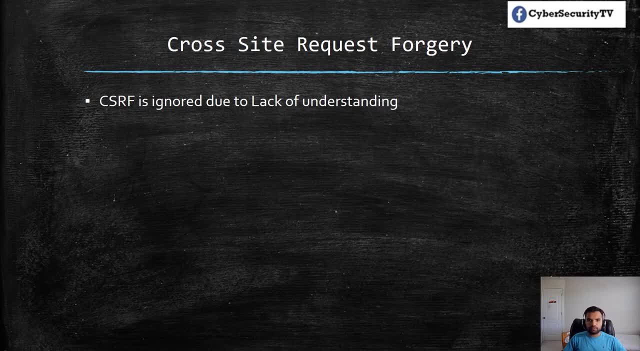 why this is important, why this is critical and why to avoid. however, it is still in the worst top 10 list, I guess, at least for past 10 years, so you can assume how any you can imagine how many websites have actually been vulnerable to cross-s YEF technologie. The attackers will only target the 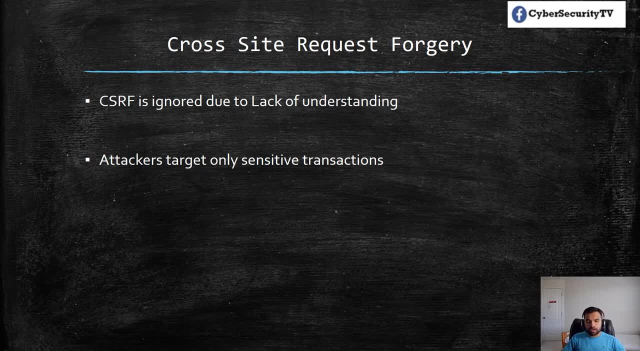 sensitive transactions. so, as I said, maybe posting a message behalf of you, maybe, like you know, sending a friend request to someone behalf of you, and we have seen this tremendous time, many people posting that, oh, my account is hacked, so don't, don't do this, uh, don't, don't reply to my message or whatever. so 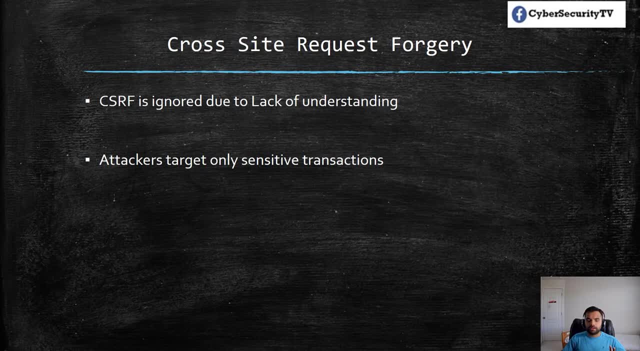 it is quite common that someone will not. uh like you know this. as i showed you the first one, someone is not going to send you like google link and click on it, and because the the attacker is not going to gain anything from that. but they might send you a link to your bank accounts or 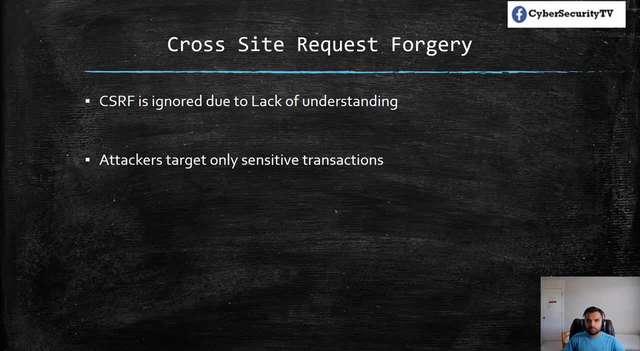 force links to your, like you know, facebook, uh, gmail or something. scanners are not going to be helpful, uh, if you are a security professional, or even if you are an engineer, developer and you want to, like you know, use some open source scanners or maybe professional scanners to scan. 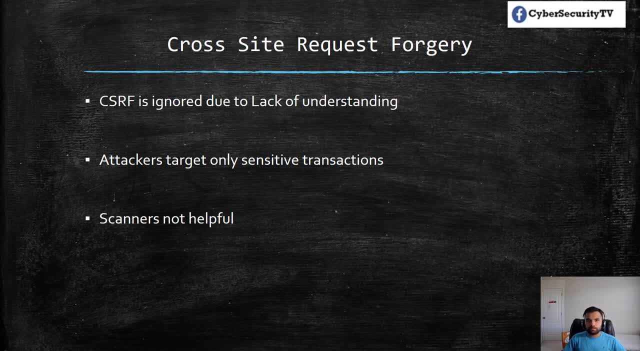 this, it's not going to be useful. even i would admit that burp is not effective on finding the cross-site request forgery issues because it pretty much like you know, uh, compare the response and see, oh, there is no token and that's why it's a csrf vulnerable. but you actually have to put the 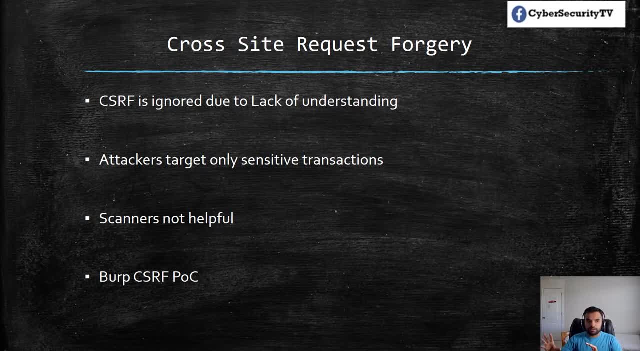 contact, you know the data to the cssrf and then you can see that the cssrf can be used to scan the of the application before you can say whether this is a vulnerable to not or not. so but anyway, let's just go back to our demo. I'll show you how exactly the 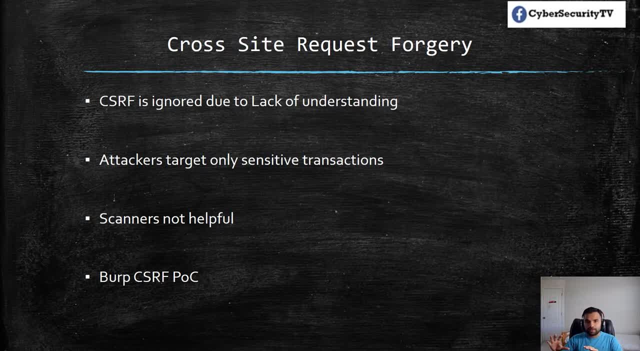 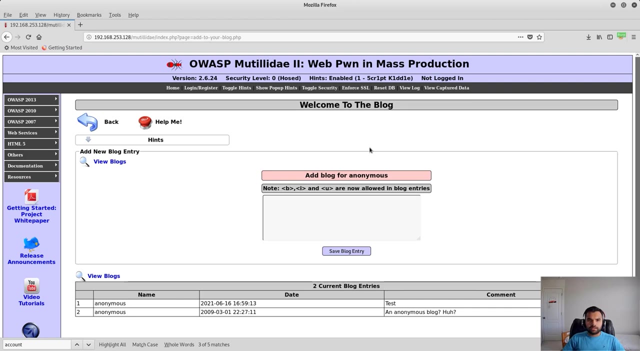 CSRF works, how you can attack the CSRF, how you can generate the proof of concept using the burp, and then, in the next video, most importantly, we will see how you can bypass the CSRF token using the cross-site scripting which you have seen in the previous video: our middle, the application, which is like an. 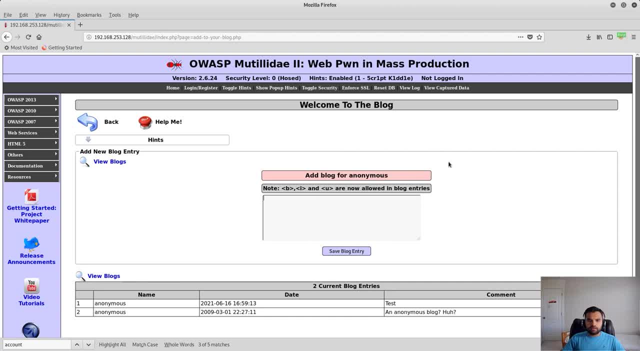 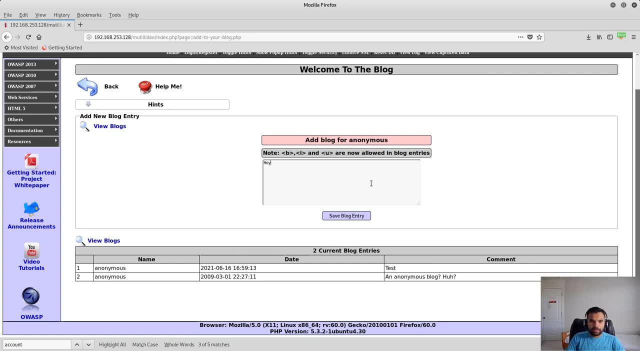 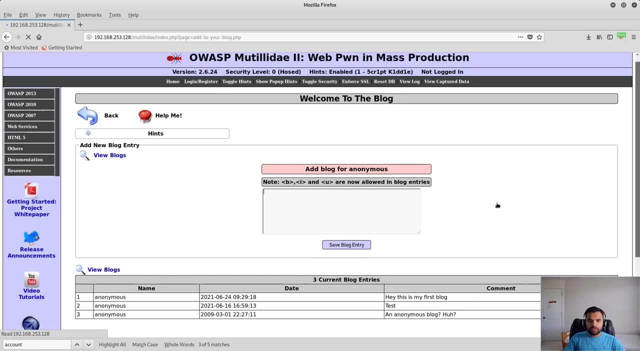 intentionally vulnerable and let's say there is. this is similar to the example that we are talking. instead of like your Facebook, we have this message where you know you can type: hey, this is my first blog and when you click on save log entry, it's gonna save it to here right now. the interesting point here to 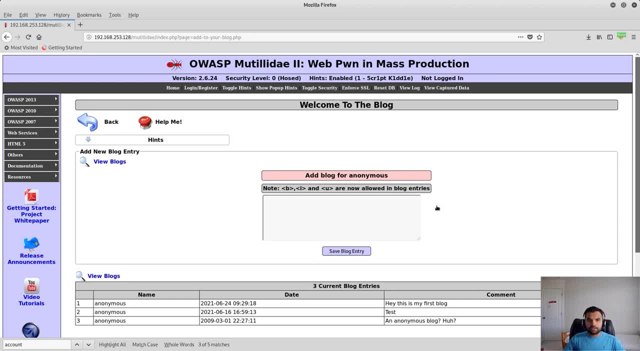 notice. how can, as an attacker, you can leverage this, like you know, attack this page and and perform the cross-site request forgery. so this is how I would like to show you that you can perform the CSRF attack. first off, make sure you have burp proxy configured. if you don't know where the foxy proxy, check it out. 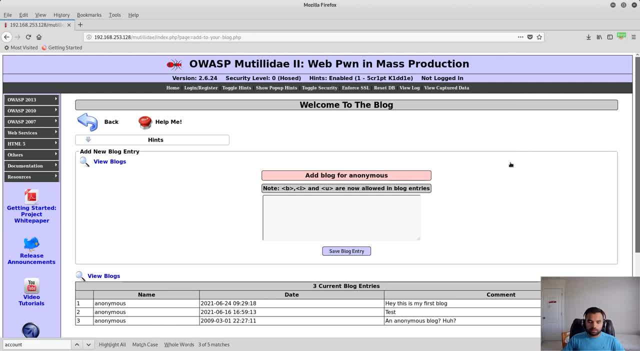 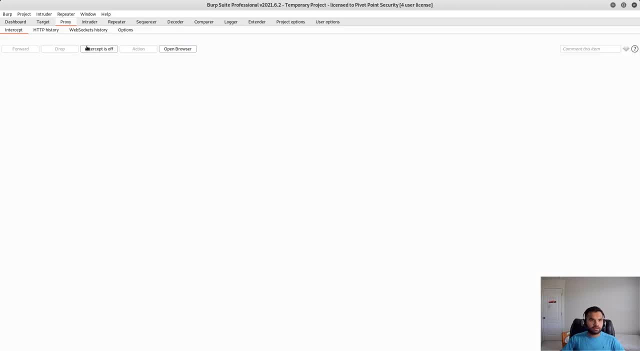 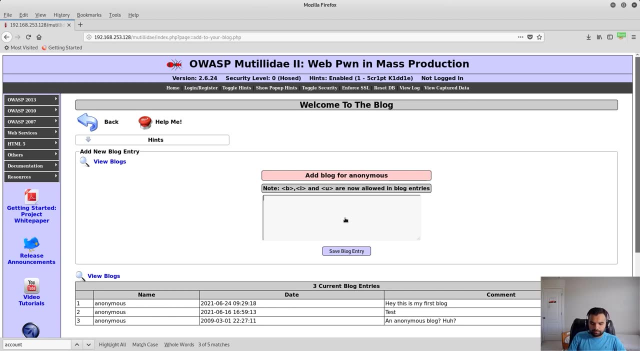 it's a really good tool, actually add-on, for navigating between different proxy. all right, this is our burp, like you know, professional edition. so what you're gonna do is you're gonna intercept on, let's say, testing CSRF, POC. okay, I'm gonna do this. of course, the request will. 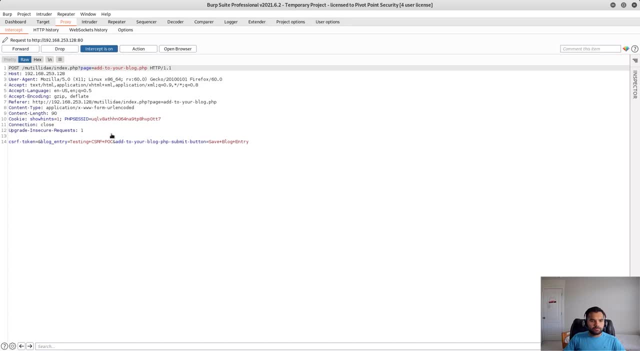 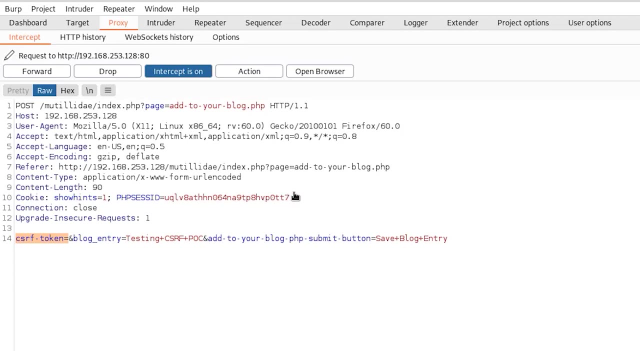 be captured here. now. one thing to notice is the CSRF token is empty. that means we can, we can easily generate this. like you know, we can easily bypass this is a like generate the CSRF POC, because there is no token. so I'm gonna do is go to the 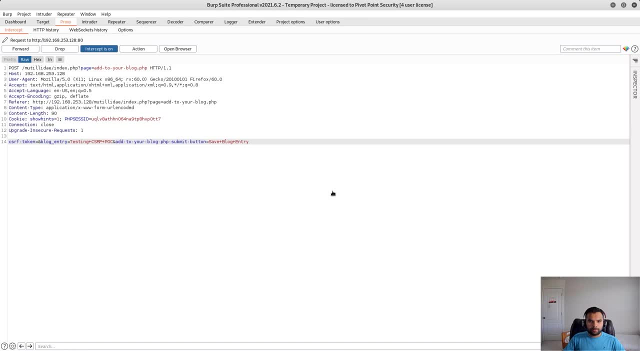 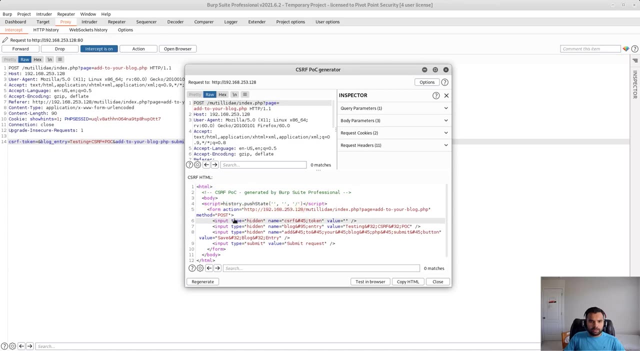 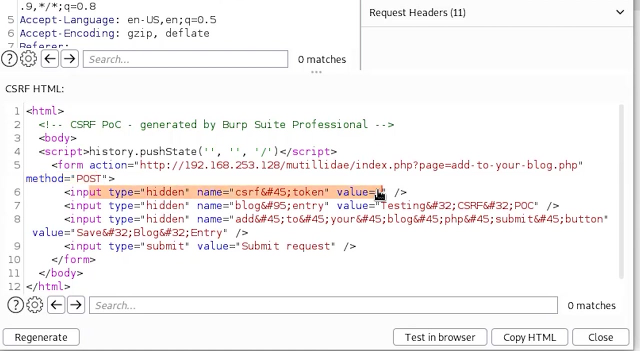 engagement tool and says: generate CSRF POC. and here, as you can see, it's a simple POC. so it says, like it, give the action and method the post. it hides all the parameters that we want to, like you know, submit behalf of the victim or the user. 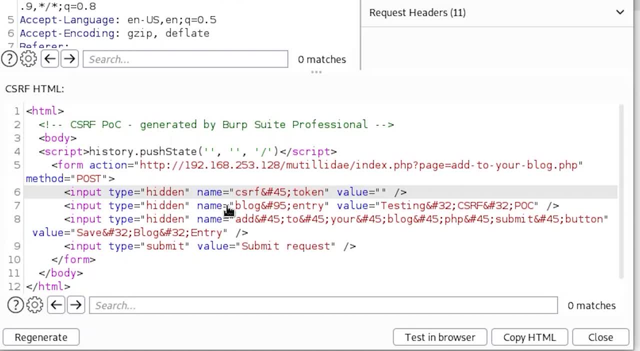 so first one is the CSRF token, which is values, M, T. then next we have the blog entry, the message itself, which is says: testing CSRF. this is URL encoded, so don't worry if you don't get it. then it says: like you know, which button do you want to click? and then that's it. so before see there. 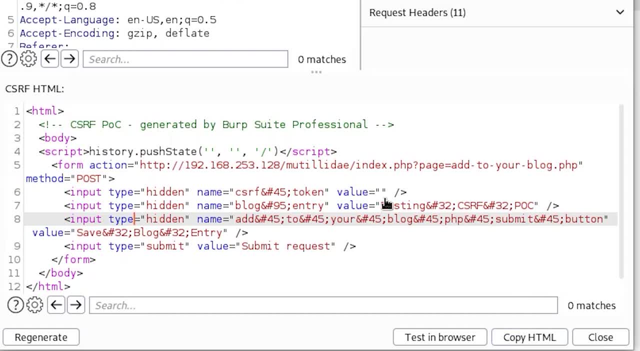 are two way you can test it out. one: you can copy the HTML, paste it in the like you know, not paid- and save the HTML and send it to someone and they click on it and it works. the other thing is you can also test in the browser. so if I say 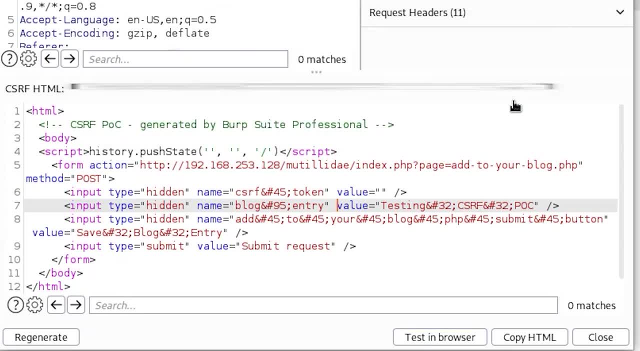 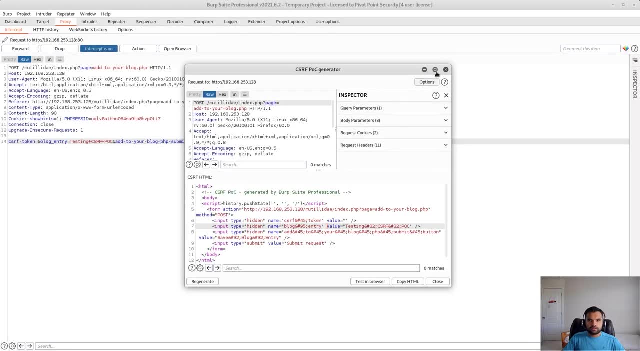 test in the browser, you can also test in the browser. so if I say test in the browser, I can copy and now go here let's say ok. before that, let me change the message so you can see successful CSRF. so testing will say success, full CSRF doesn't. 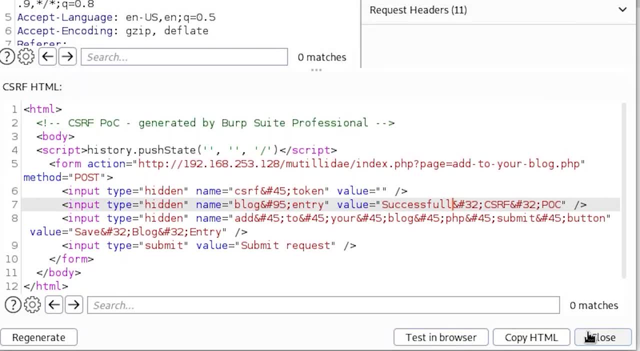 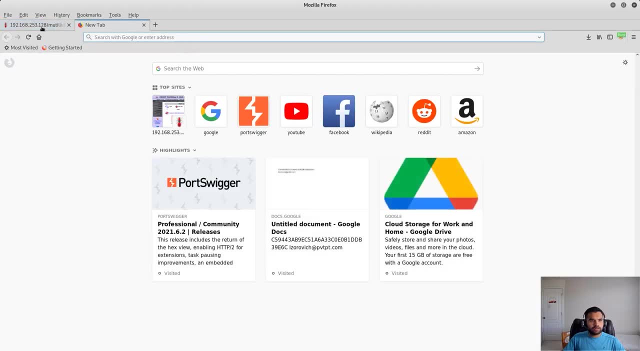 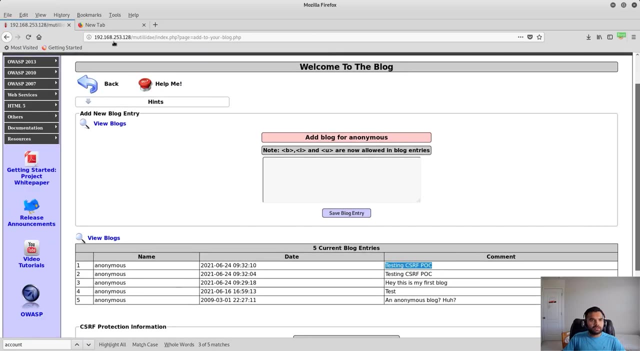 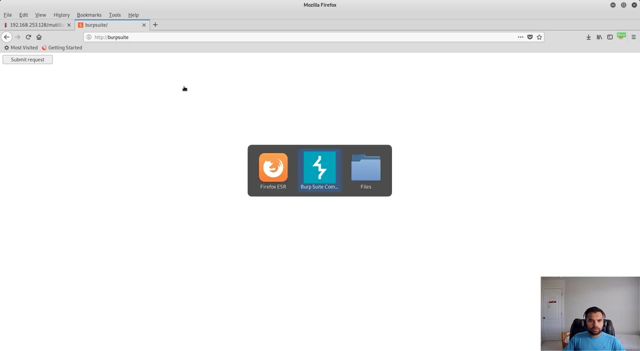 browser copy: close, intercept off. ok, let's go here. so now, if you see here present, it says testing CSRF POC right now. this was the link which was given by Bob. alright, so this is the same page that we saw, the code here when we were generating the POC. right, there is nothing difference. you can also do it in. 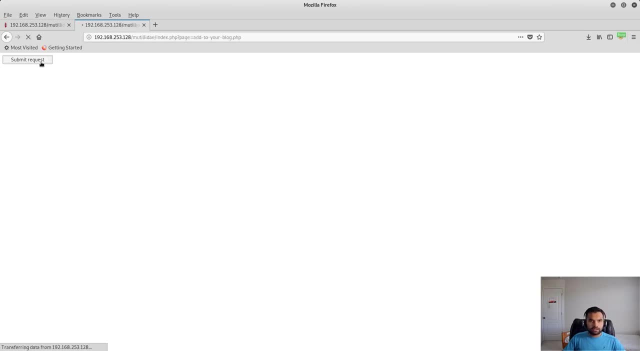 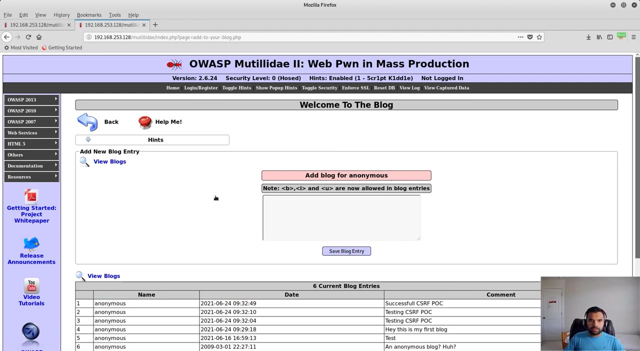 the HTML and you can open the HTML page. so as soon as I hit the submit request, you can see successful CSRF POC. now, of course, in the real world scenario it won't be the same browser, it will be different users, but the logic remains the same: once you send this HTML to someone or link to someone, 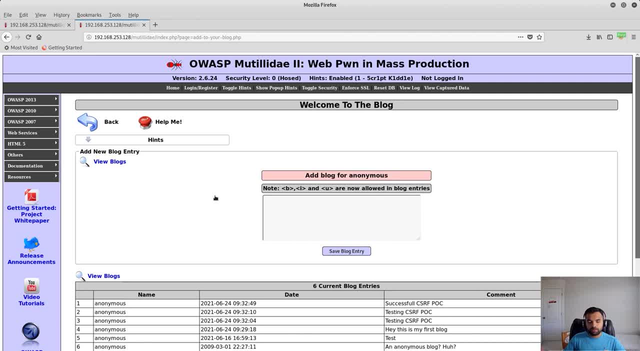 they click on the submit button. even sometimes they don't have to even click on submit, but you can auto medically click on behalf of the user. so user doesn't notice anything and it will pose the message behalf of the user. now how? how generally developer prevent that. so the 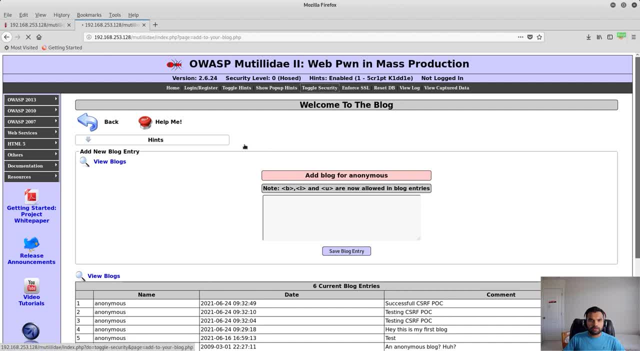 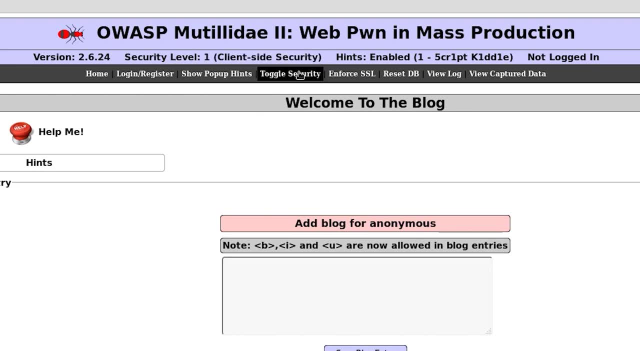 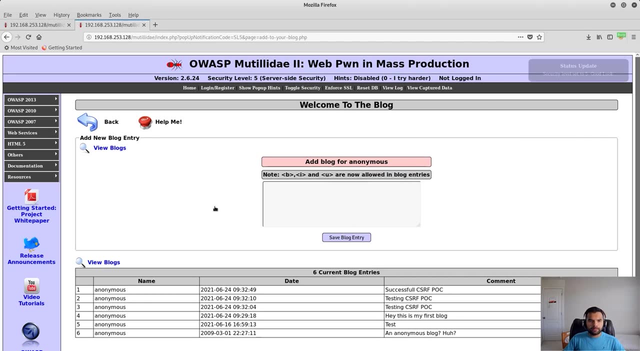 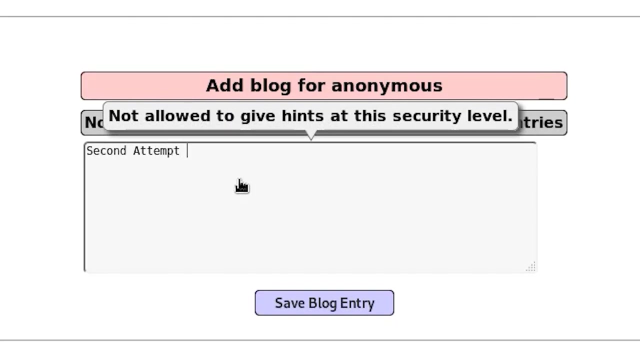 easiest ways to prevent it is: let's talk with the security here. so now you can see a. the security is one. actually, you can again toggle the security. let's say server-side security. okay, so this is the highest security that you could get. now let's intercept again and say second attempt, or CSRF, save blog entry. let's go. 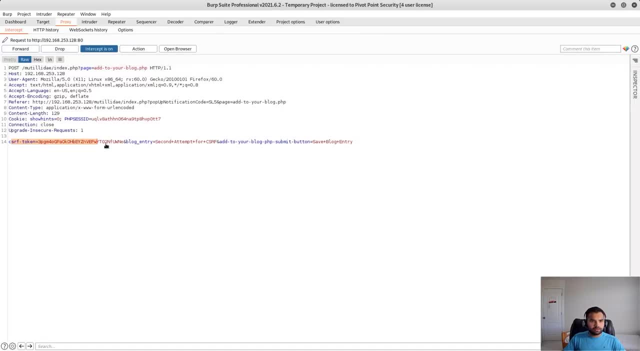 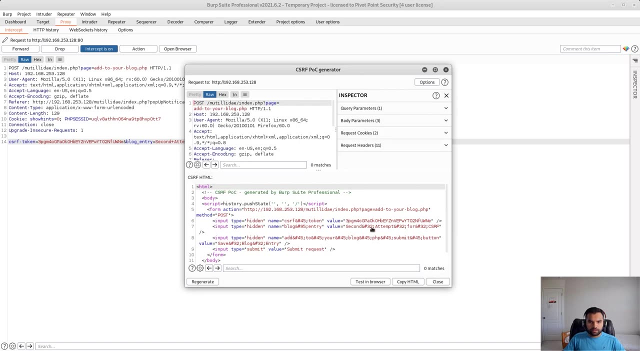 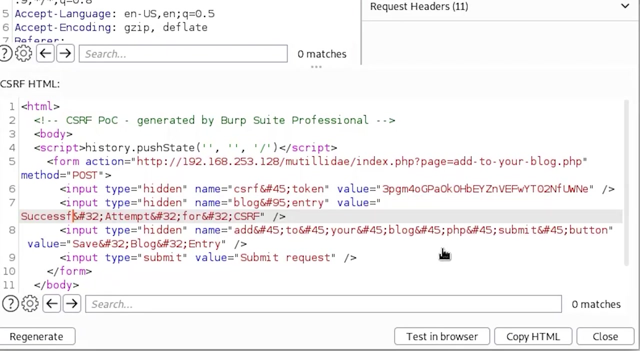 here. you can see now the CSRF token is right here now. if you are so, for example, let's say, when you generate the CSRF POC, right, you'll have this, and this will say second attempt. I'm gonna say successful, second attempt, second attempt for CSRF. okay, now one thing you would notice this time: 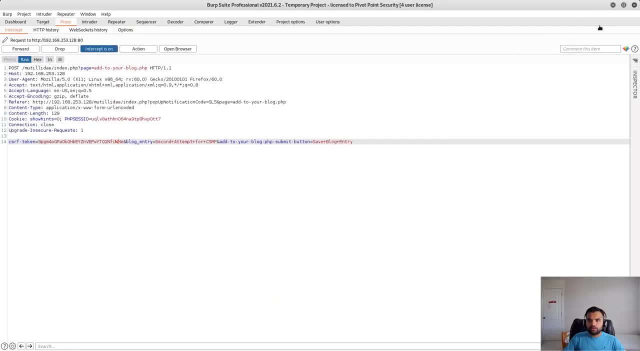 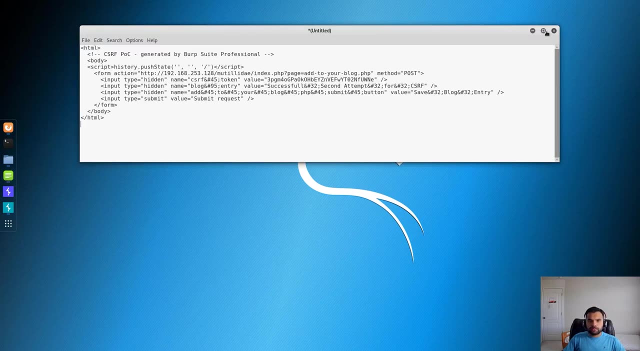 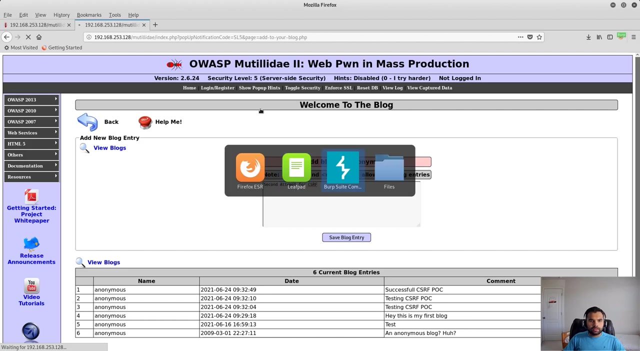 I'm gonna let's copy the HTML because I want to show you something. let me open up the lift pad, paste this here and let's just keep it here. so just notice this CSRF token right now. of course, if I turn this intercept off, it's gonna say second. 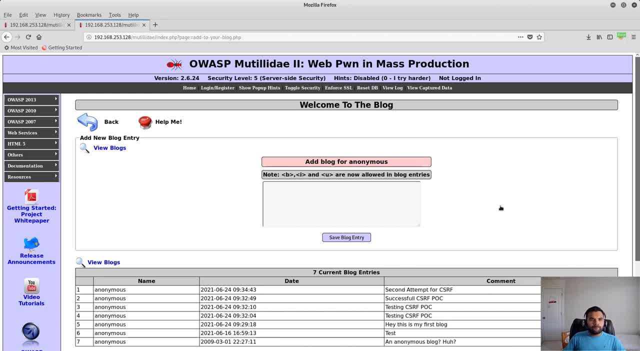 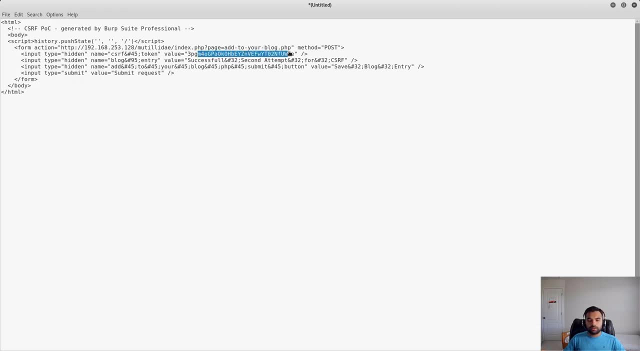 attempt for CSRF right here, right now. in the usual application, when the user logs in, each user will have the different token. so here the token that you have got might be different from the token that you are trying to export the user for right. so the I, as a user, a, might have a. 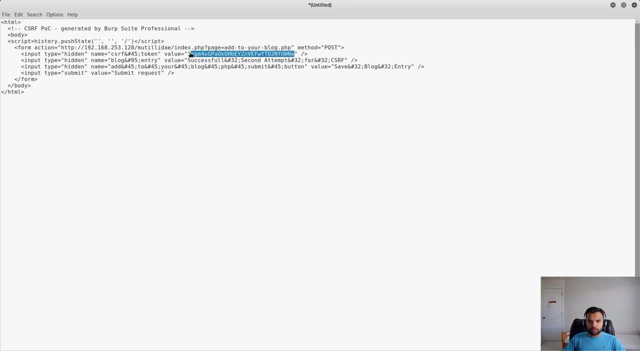 different token, like, might not have at the same value as this one. so if I send the same value, let's say my value is different and and you're trying to change it, and I just put some random numbers here and now, if we try to submit this, it's not gonna work. why? because this token does not work. if we try to use contents like semultum, now thiskin. 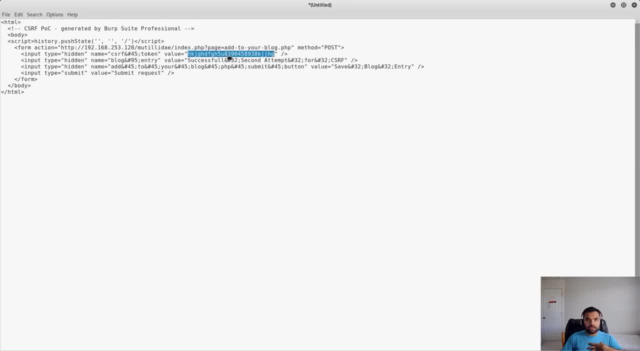 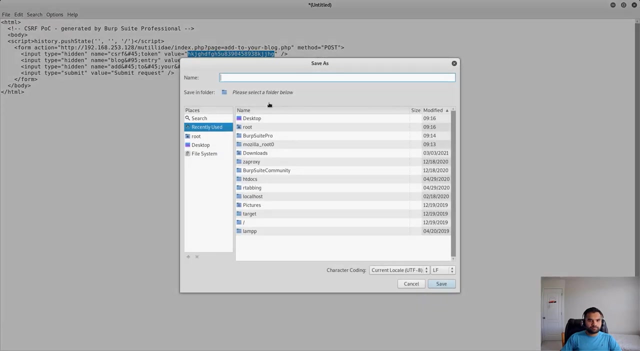 does not be vi as an attacker. do not have user a csrf token which was given to him when he or she was logged in, and that's the main way to prevent the csrf, right? so so let's just try this. uh, let me save this file. i'm going to save it on the desktop and say: csrf poc dot html. 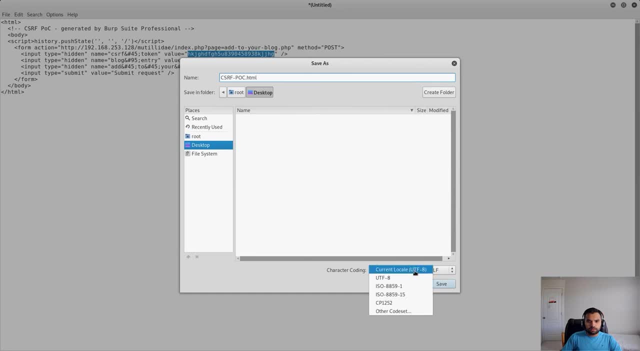 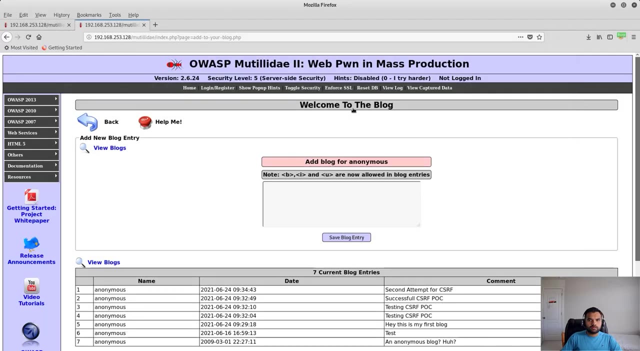 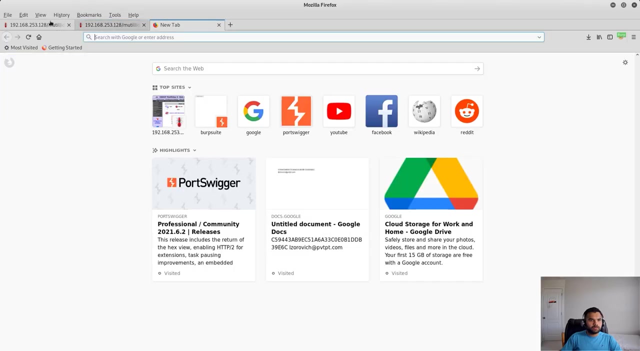 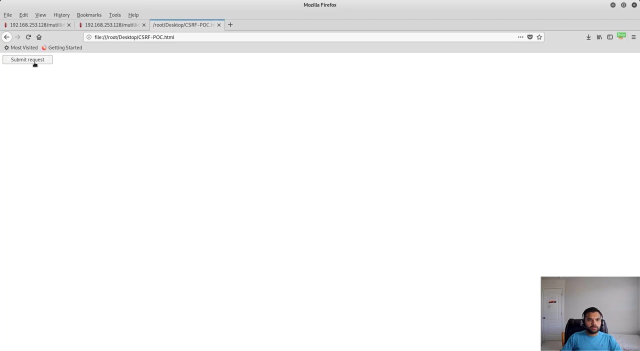 okay, save, save, okay, and let's open this up. file: open file: csrf, poc. right, it's gonna say submit request. if you see the source code, it's the same one that we just saw. of course i i intentionally changed the token, uh, but of course i as an attacker do not have any control if i'm in the 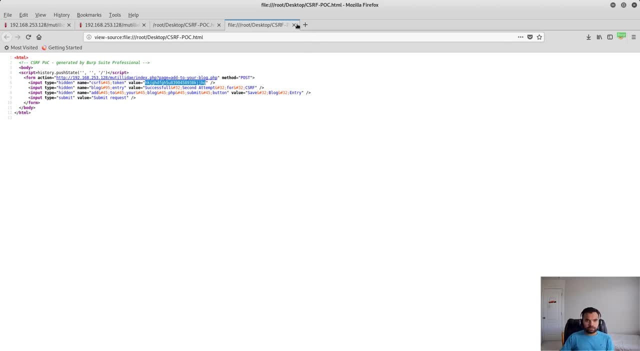 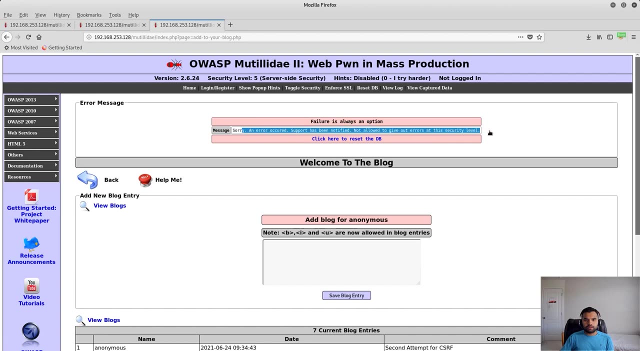 real world scenario. i don't have any control on what the user's token is, so i'm gonna submit this request. it will say: sorry, another support has been notified, not allowed to give it out. error at the security level and, as you can see, the second attempt of successful csrf uh did not work. 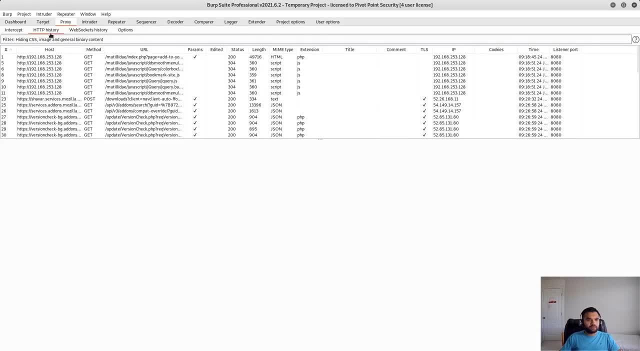 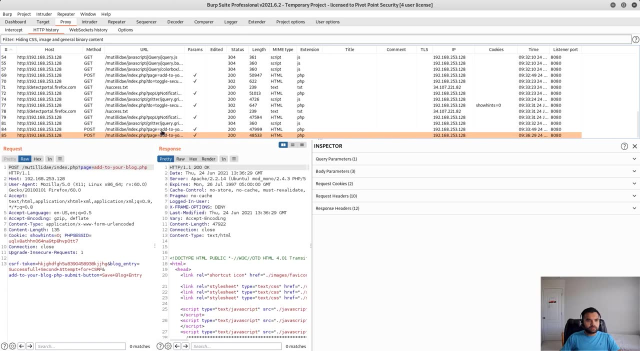 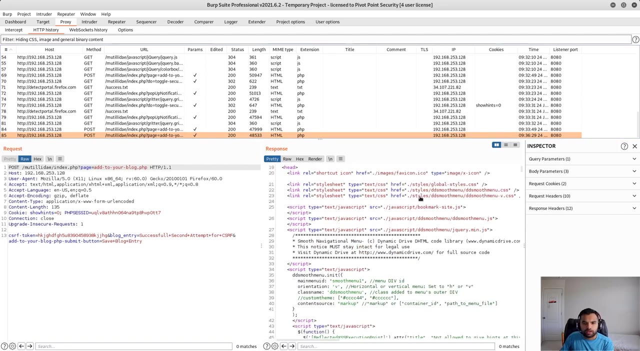 so maybe if we check out here, right, this one, i don't think say if it got logged or not, but yeah, i think this is the one, yeah, this is the one, and, and you can also see, like the: okay, here we cannot see the error page, but yeah, you can easily. 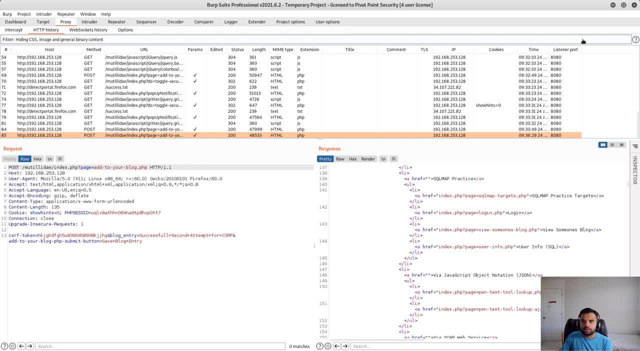 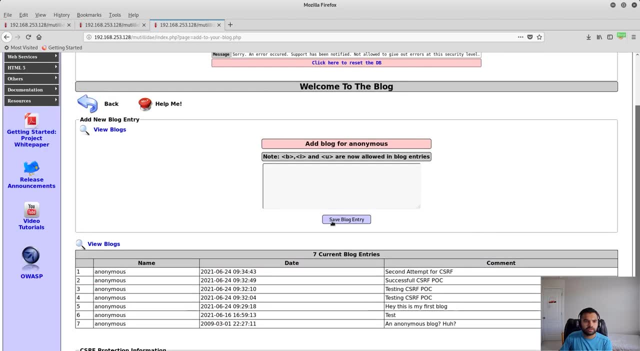 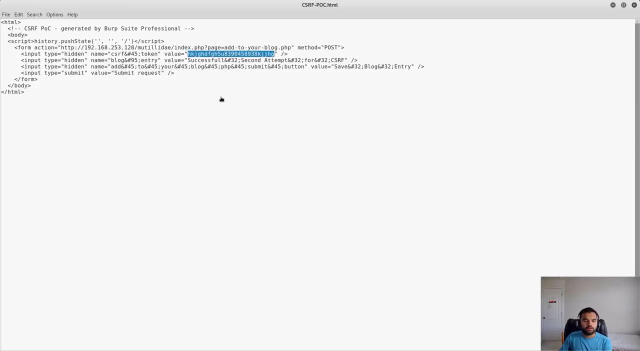 search and and our payload did not get executed. and if, even if we refresh here, yeah, successful csrf poc did not come through and the main reason was because we had this. uh, main reason was that we could not guess this token of the user now as an attacker. how, how would you guess it? like? 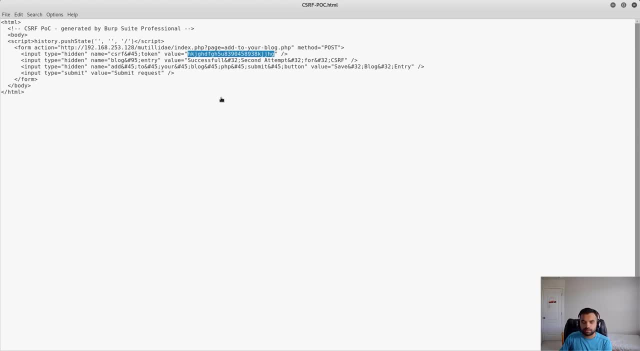 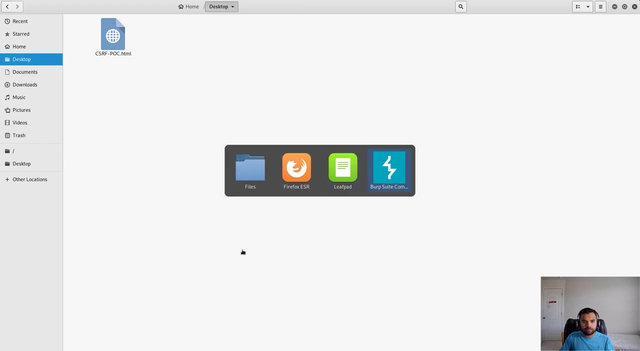 how do you bypass this? there is no physical like. there is no literally way to do this like without asking a user to send this token, because this token is in the hidden value, like the when, when you saw the request in the burp, like for the valid request, uh, the token is not in the cookie. a cookie. 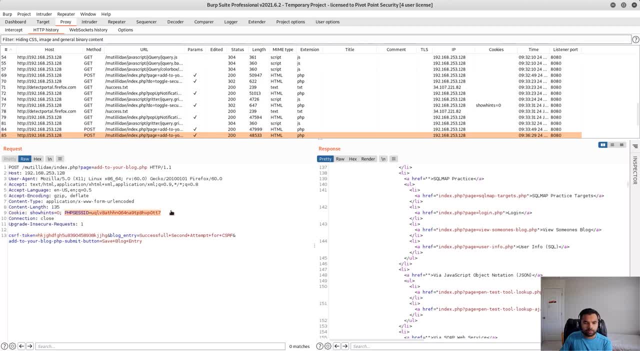 automatically by the browser, so we don't have to worry about, like, guessing the cookie value. but this value is sent in the request body, so we have to guess each and every value correctly before we can proceed our attack. so this is where we are stuck. the next week is going to be very 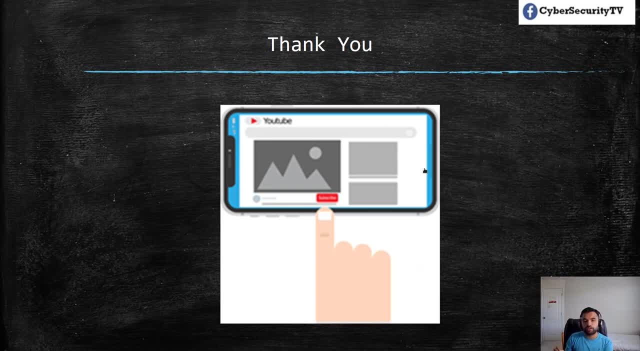 very interesting because i'm going to show you how you can leverage ajax and the process scripting to steal the csrf token, which is random, and, and you copy the token and attach into the csrf request, you generate the poc and then you submit, no matter how strong the csf token is. so it's going to be very interesting. 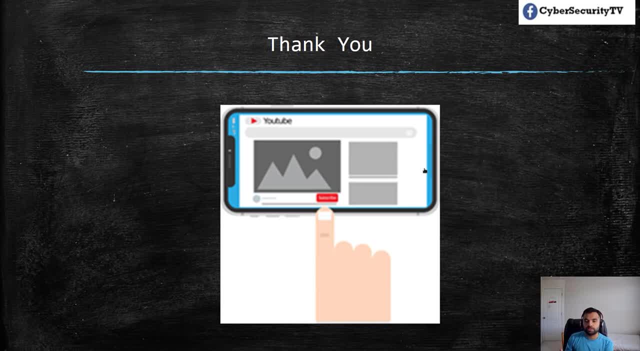 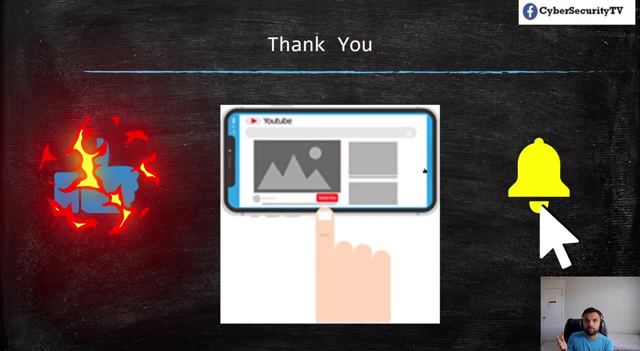 so stay tuned for that. if you have any questions in the interim, feel free to drop it down in the comment section. i hope you like it. please hit the thumbs up button. if you do subscribe to my channel, follow us on the facebook so you get the latest updates. i'll see you guys next week. bye.